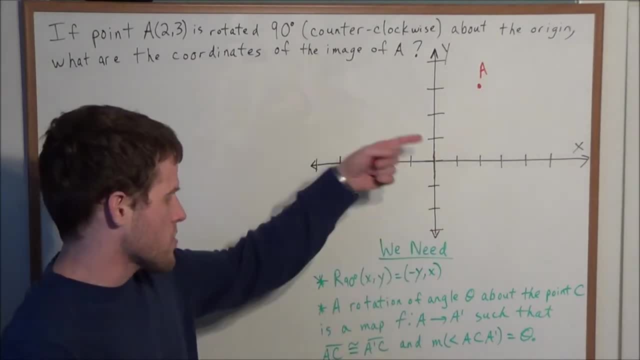 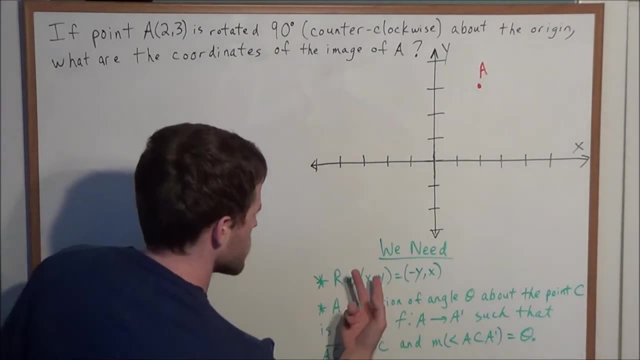 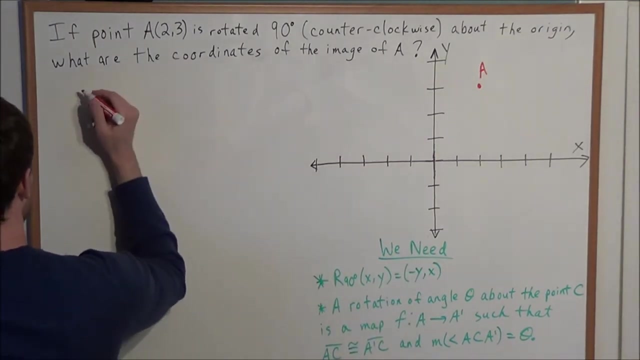 a point and we rotate it 90 degrees counterclockwise, about the origin. this point gets mapped to. So all we need to do is swap the x and y coordinates and negate the y coordinate. So if we apply this definition to, we have a rotation of the point. 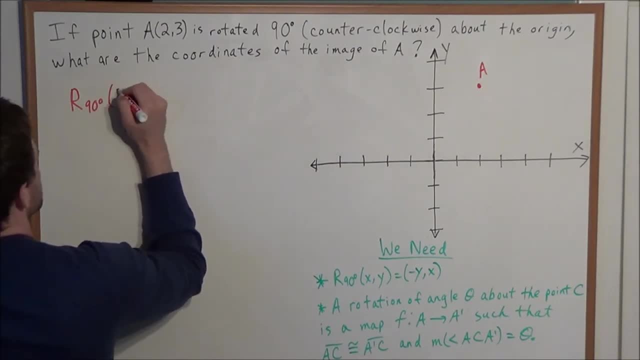 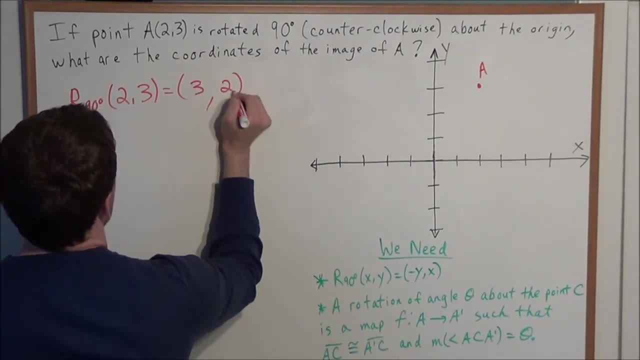 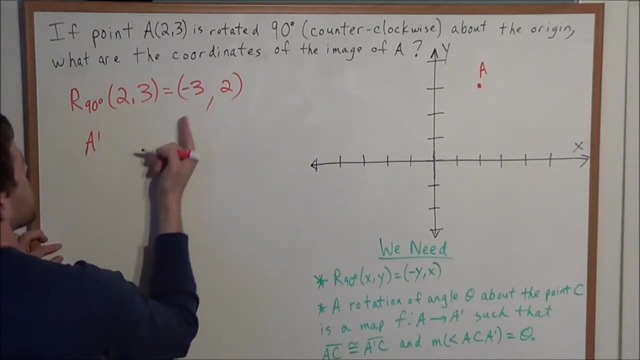 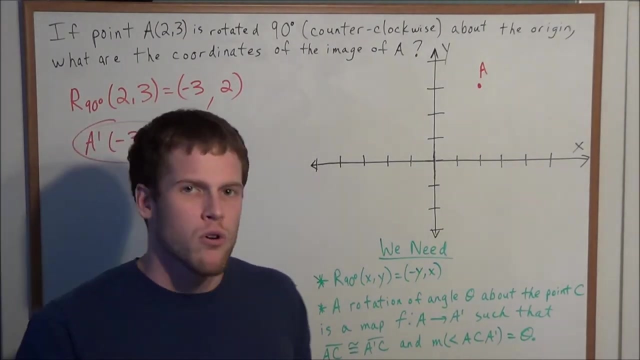 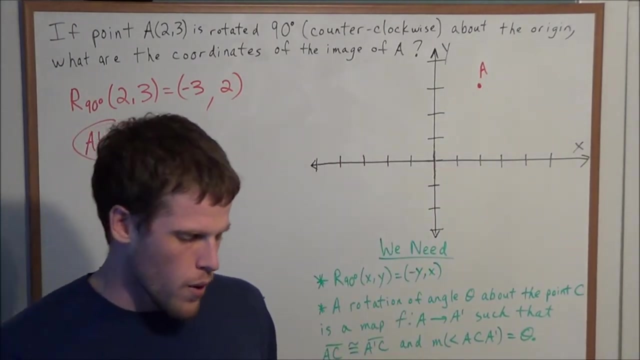 90 degrees counterclockwise. So the image of A- we can call it A prime- will be the point. But now this doesn't really say much about what a rotation is. So the second method for solving this problem would involve using visuals. So if you have the point plotted on your screen, you can 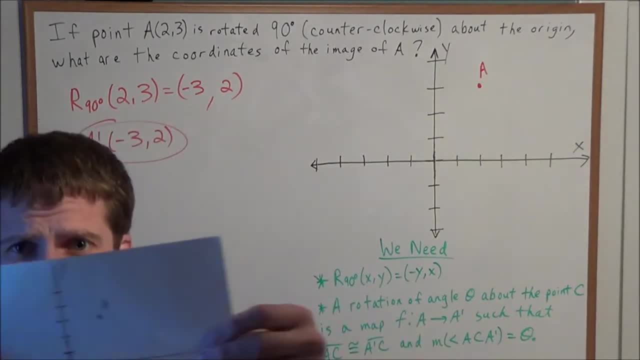 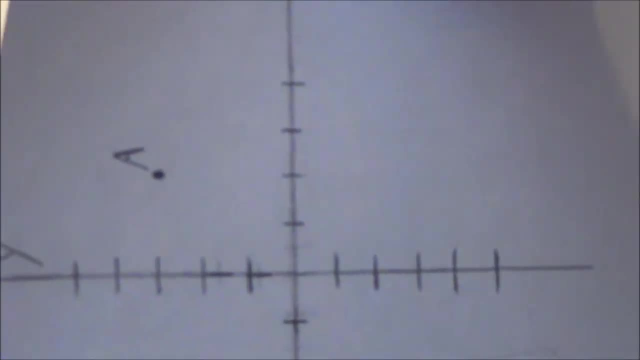 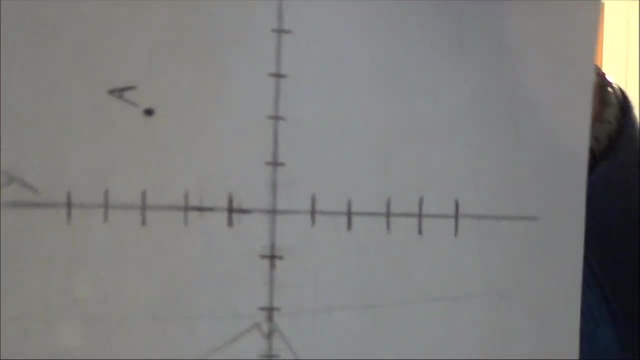 see on your paper the point. You could physically take your paper and you could rotate your paper 90 degrees counterclockwise. And now, where does A get sent to? Well, it goes to the point. So by taking your paper and rotating it 90 degrees counterclockwise. 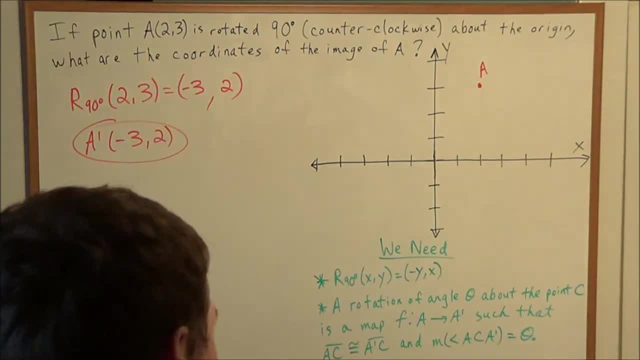 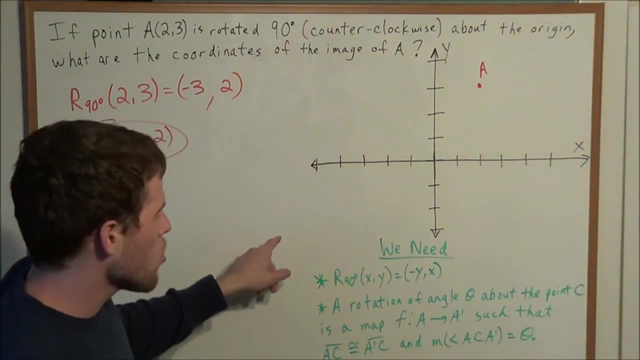 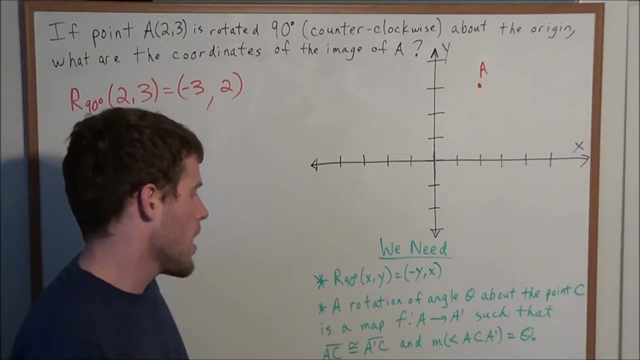 this is a second way of finding the image of A. Now the third method for finding the image of A is a little bit more complicated, but this would be a little bit easier to do. So let's look at where this equation comes from. So, when we have a, 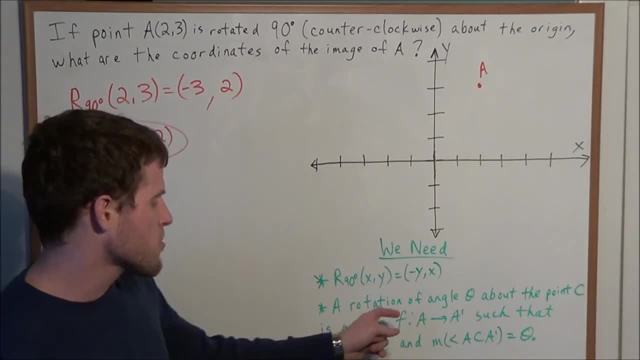 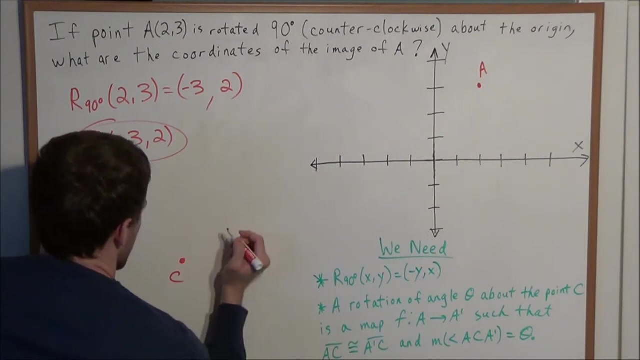 rotation. let's look at the definition A rotation of angle theta. about the point C is a map from A to A prime, such that the length of line segment AC is congruent to the length of line segment A, prime C and the measure of angle ACA prime equals theta. So all that. what this means is we have some center. 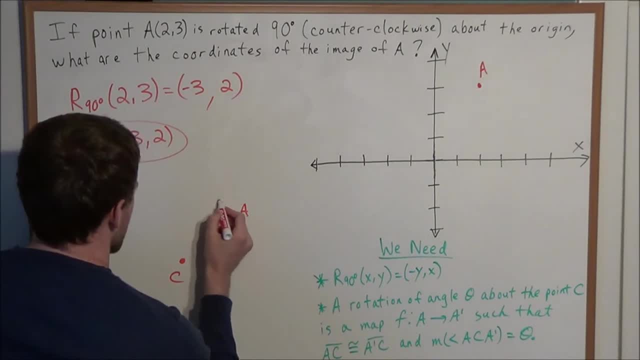 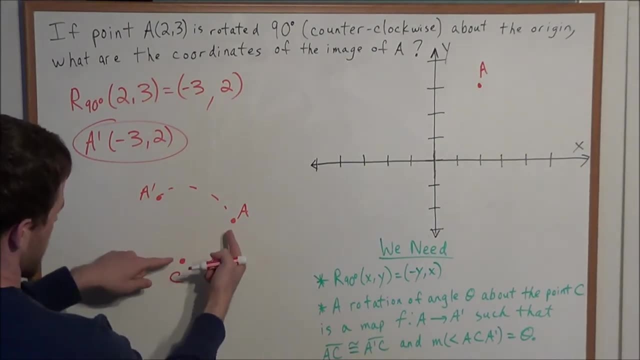 of rotation C and some point A To A prime. let's say we rotate A theta degrees about the center. This means that angle A, C, A prime is theta degrees and the length of line segment AC is congruent to the length of line. 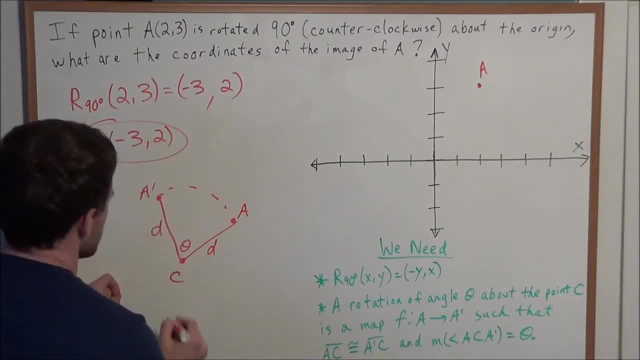 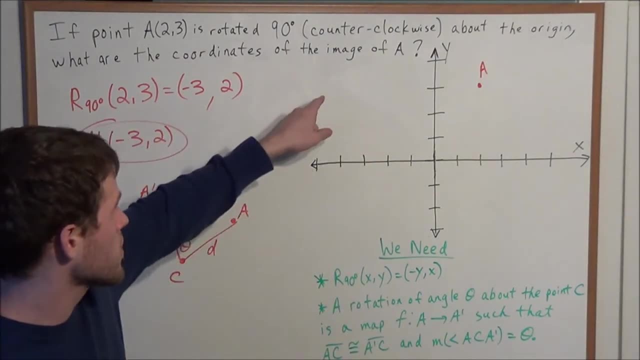 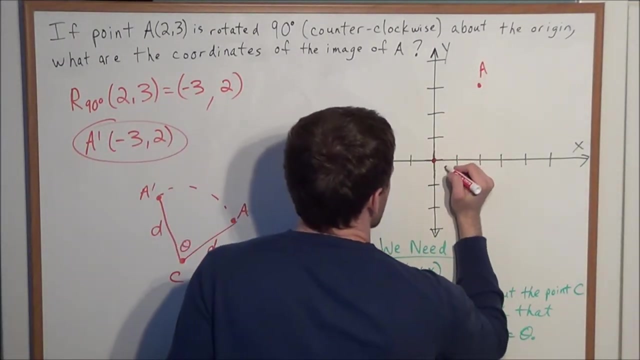 segment A prime C. So that means that these two would be, let's say, D units long. So this is really just a visual to accompany the definition of A rotation. But now, how does this help us find the coordinates of A Inside point, A prime? Well, if we're fixed at the origin, we can fix a point at the origin. we'll call this. 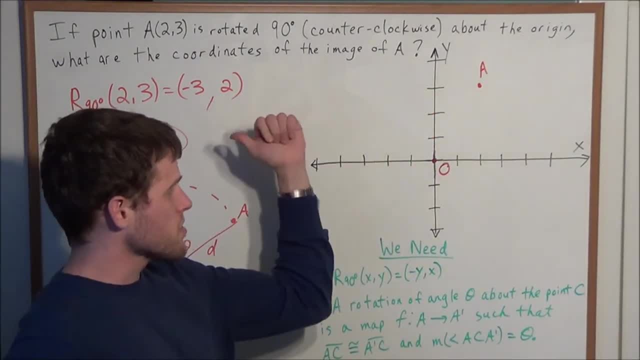 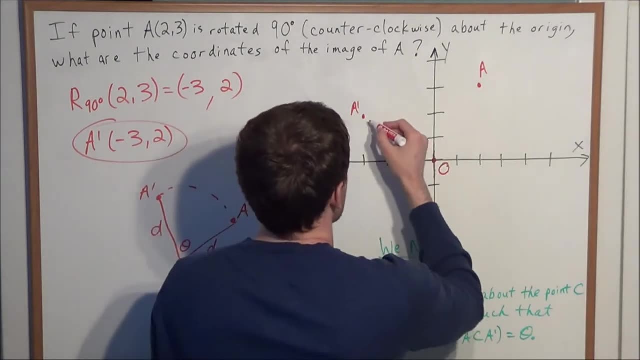 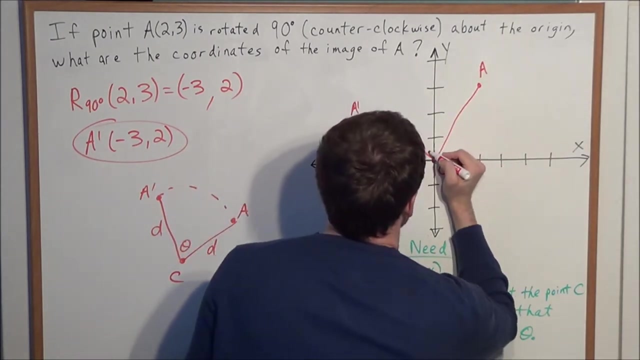 point O and we're rotating A 90 degrees counterclockwise. well, this is gonna send us to the point A prime, and there's gonna be two conditions that are filled. Angle AOA prime is 90 degrees, since it's a 90 degree counterclockwise. 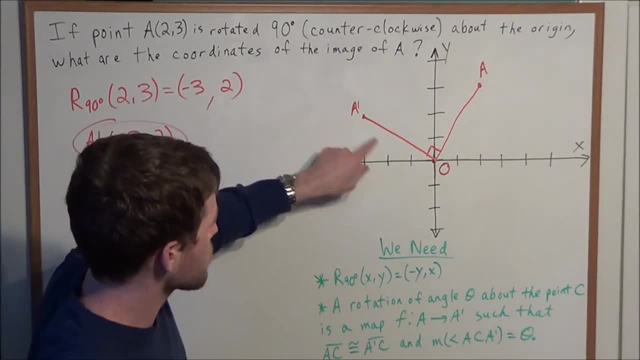 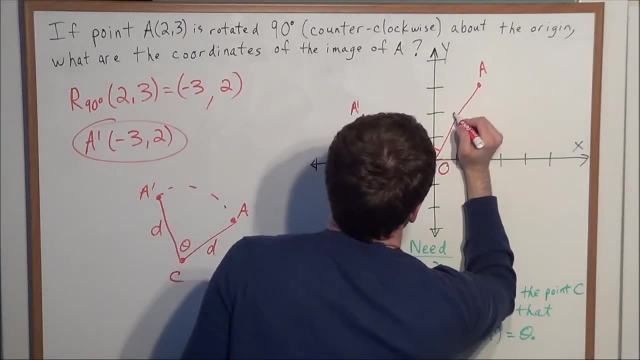 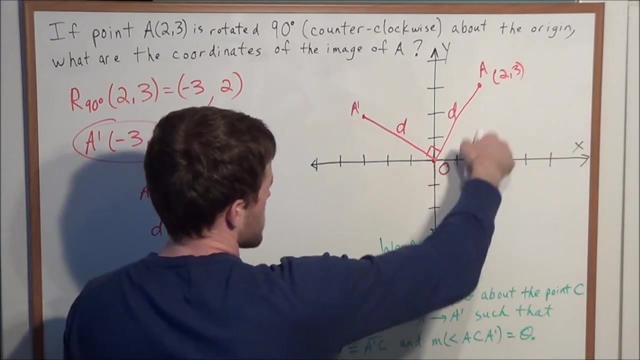 rotation and the� line segment A prime O is equal to the length of line segment AO. So we have, let's say they're D units long, But we do know that A is located at the coordinate. So if we want to trace a path to A, we're going a horizontal distance of 2. 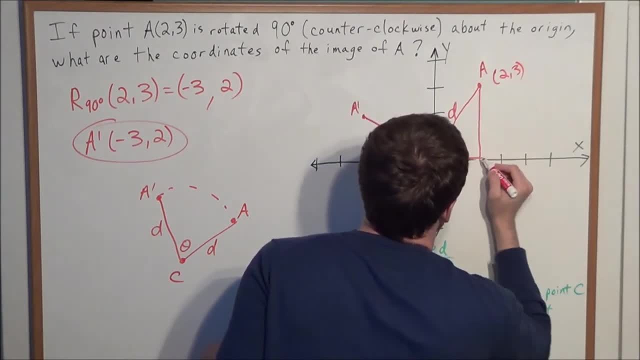 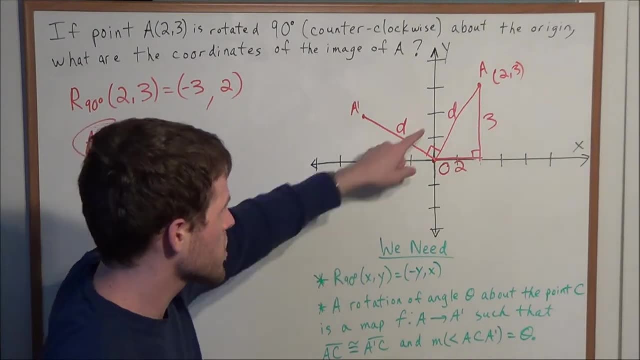 and a vertical distance of 3.. But when we trace this path, we're creating a right angle, So we just created a right triangle. We could find the length of D, but it's not important for showing the coordinates of A prime. So now let's. 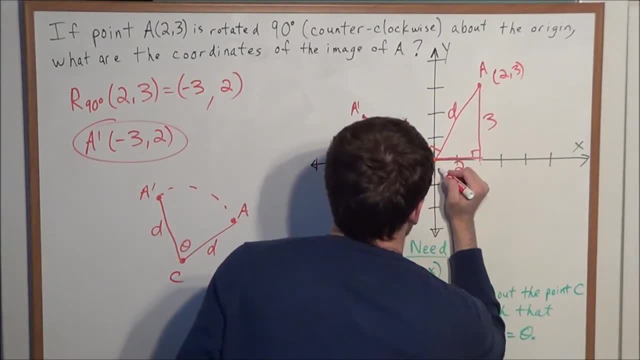 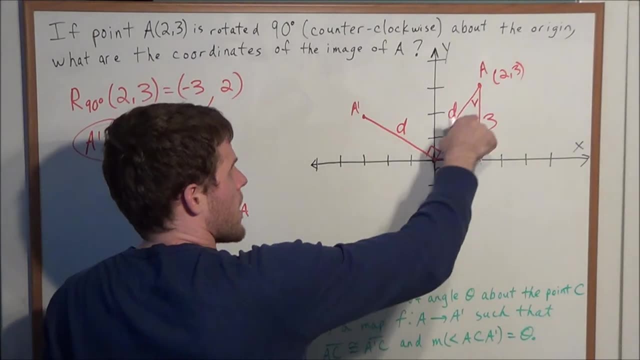 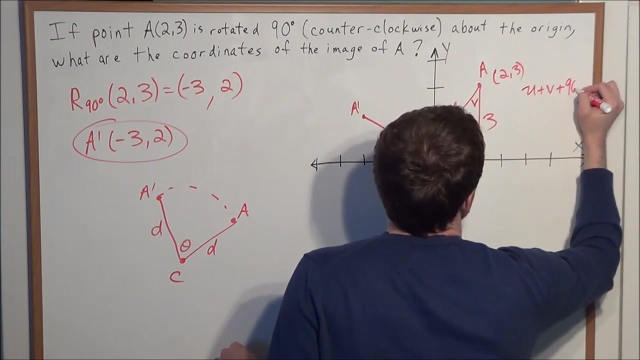 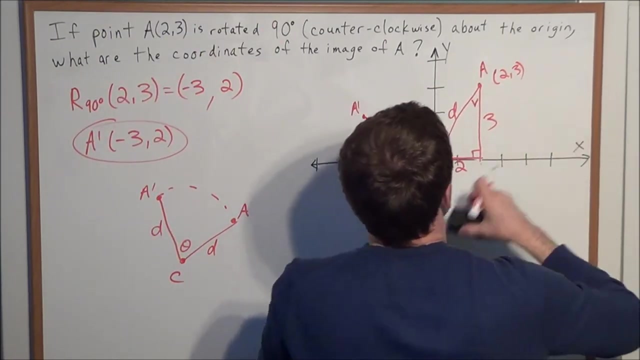 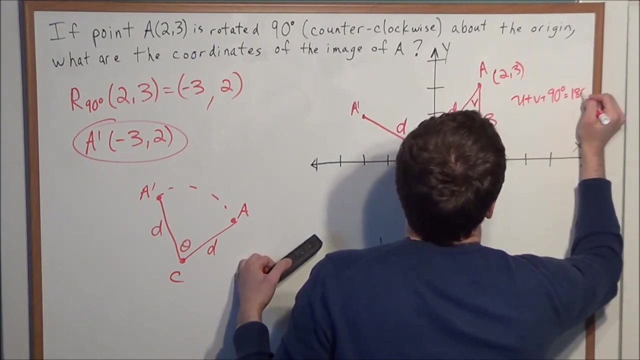 label the other angles inside this right triangle. Let's say that this is angle U and this is angle V. Well, what do we have? We have that U plus V plus 90 degrees is equal to 180 degrees. So I'll write this out a little bit neater. So we have: U plus V plus 90 equals 180.. 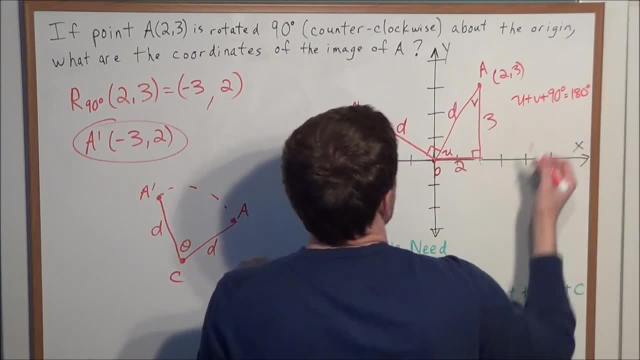 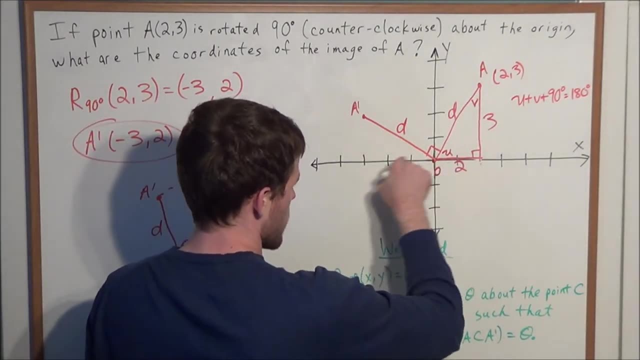 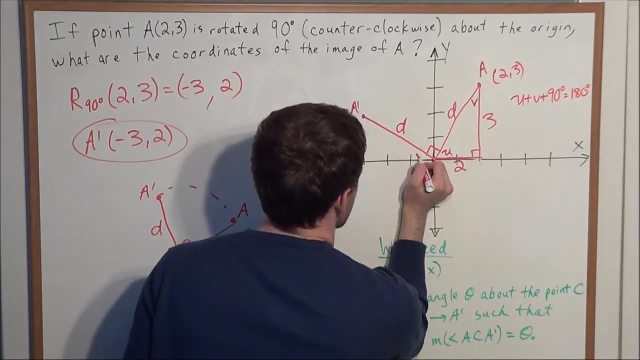 Remember, degrees, degrees. So now, what does this tell us? Well, this missing piece. here, on a straight line, we also have 180 degrees. So we have a straight line along the x-axis and we have angle U 90. So this angle here has to be V, since we already determined. 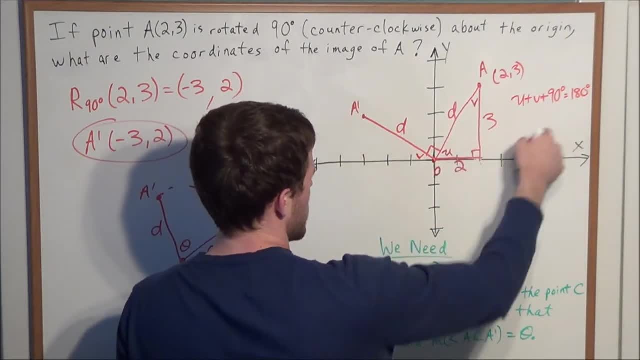 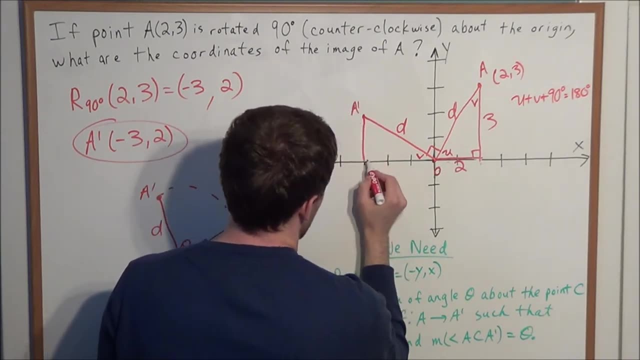 or we set U plus V plus 90.. 90 equal to 180.. So this angle here has to be equal to angle V. So now, when we draw a right triangle to the point A prime, what is this missing angle here? Well, we have 90 degrees. 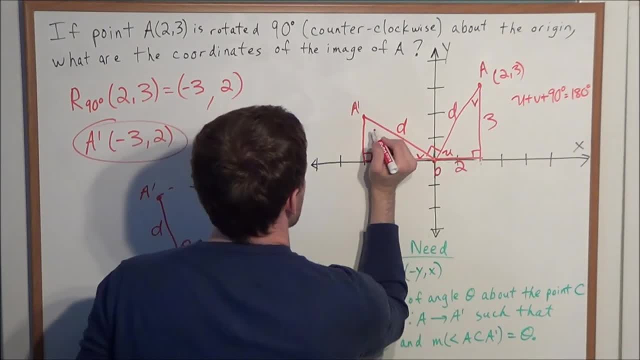 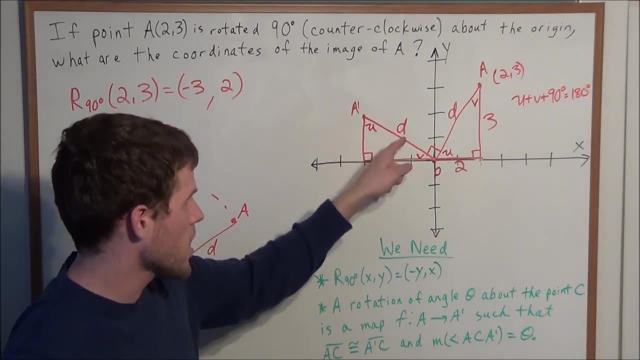 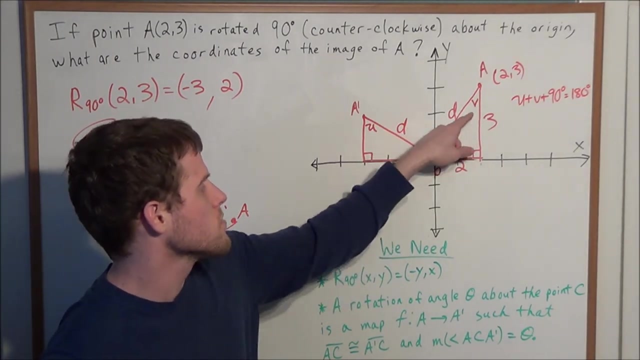 We have V, So this missing angle has to be U, And now we have two congruent right triangles, since they share the same angle-side angle: Angle U side length, D angle V. Angle U side length, D angle V. So, since these two triangles are congruent, from angle U to the